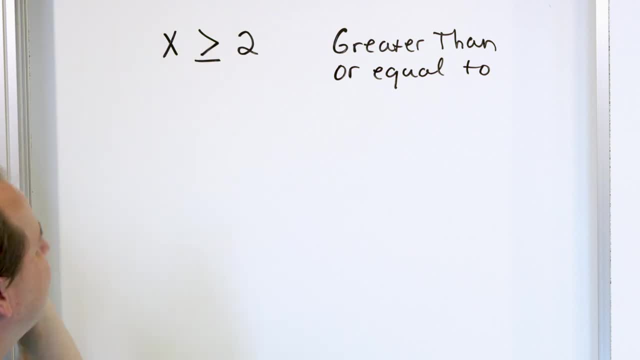 2 or larger than 2 is what x can be. So 2 can be 3,, 4,, 5,, 6,, 7, all the way up to infinity, because it just has to be larger than or equal to 2.. It can be any number. It could be 100. 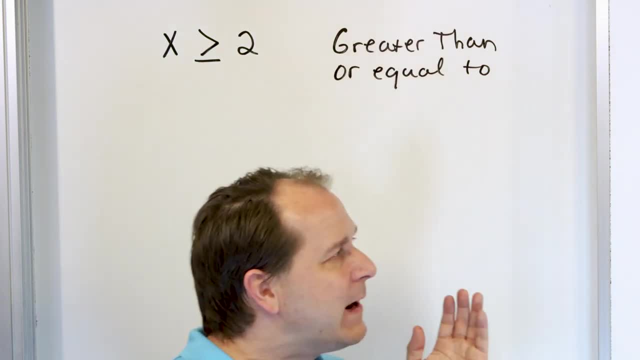 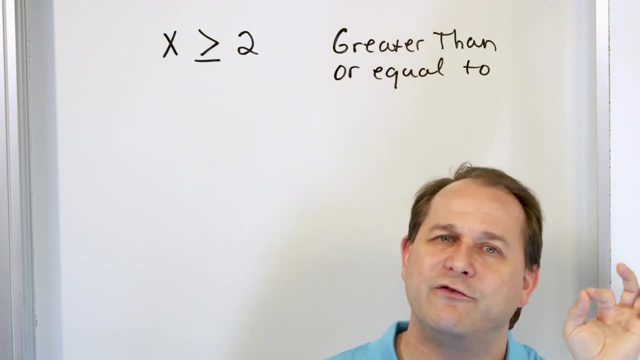 million, anything bigger than 2 or equal to 2.. Now remember the numbers here that go into. x can be any number, They can be decimals. That also means that any number that is larger than 2, even tiny little fractions or decimals, are included in this as well. So for instance: 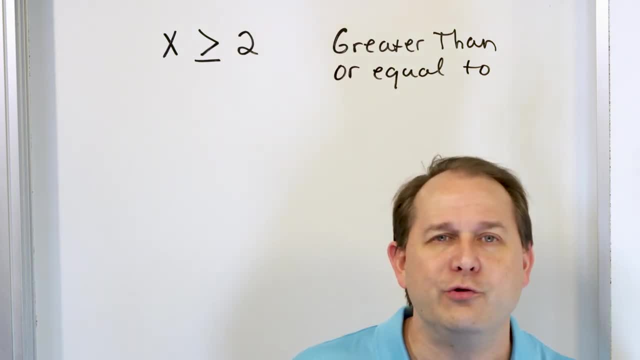 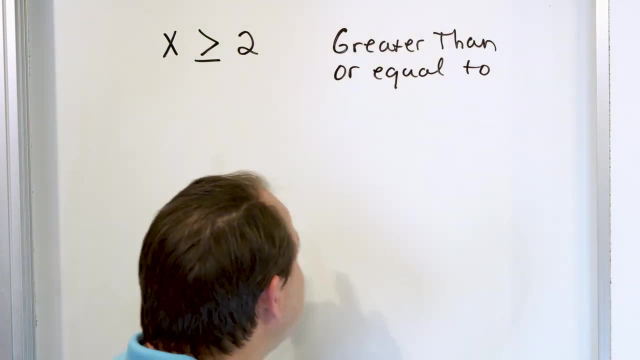 2.1,, 2.0001,, 2.0000001,. right, That's just a tiny bit bigger than 2.. And so it also satisfies this as well. So any number bigger than 2, greater than 2, or equal to 2.. Now I want to show you. 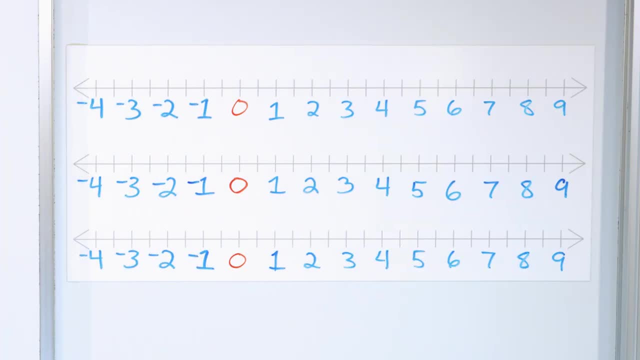 that typically, what we do when we graph these inequalities is we put them on a number line here, And so what we're going to do is we're going to put them on a number line here, And so what we're going to do in a minute is we're going to solve an inequality. We're going to use the rules of 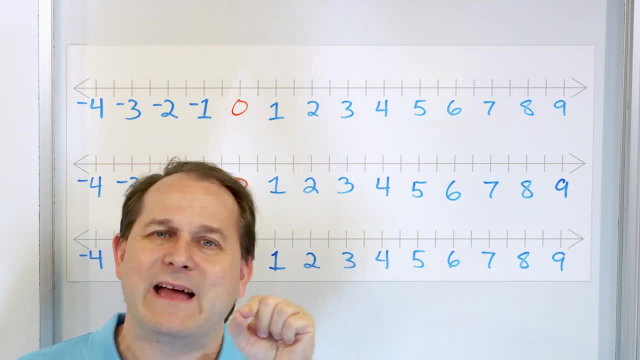 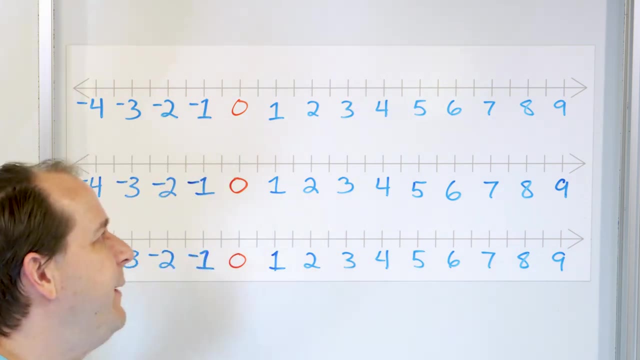 equations to solve for the values of x, But we're going to have that inequality symbol, So the answers we get will always look like what I just wrote on the board: greater than or equal to- And we always want to draw a picture of that. So, for instance, if I was going to represent this guy, 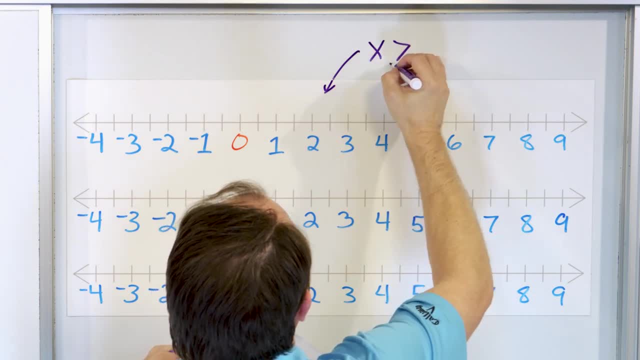 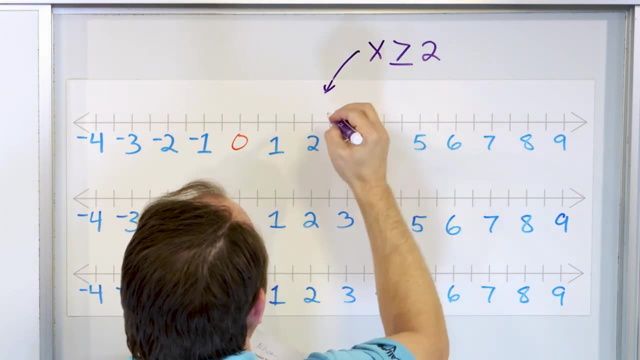 I'll just kind of draw a little arrow here. Remember what we wrote down is: x is greater than or equal to 2.. I'm just reminding you what it is right. What we are saying is that if it was just x is equal to 2, we would just put a dot on the line. That's what we would put here, because 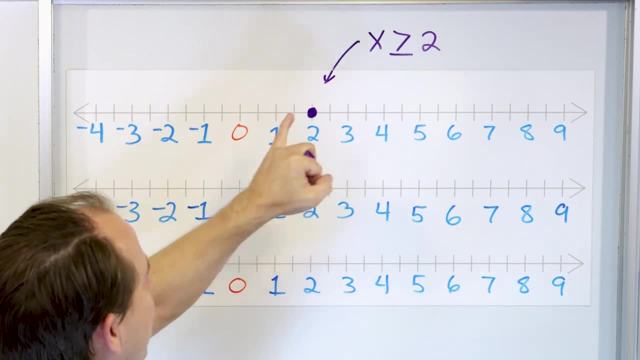 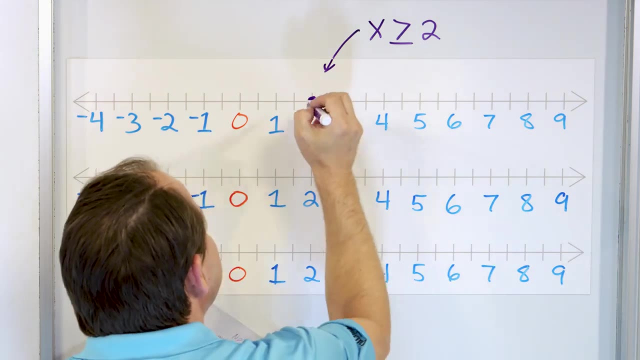 the dot on the numbered line is where x is equal to 2.. But we're not saying that x is just equal to 2.. We're saying it's equal to 2 plus any other number bigger than 2.. So what you do is you put a. 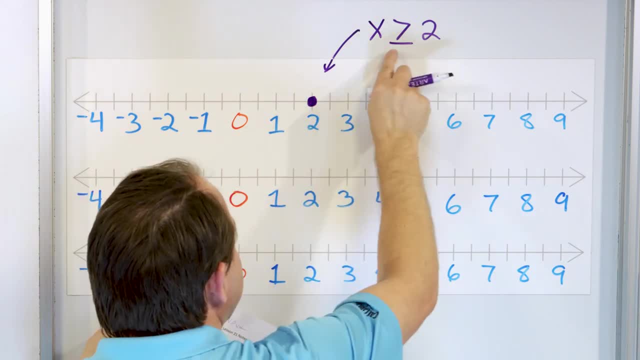 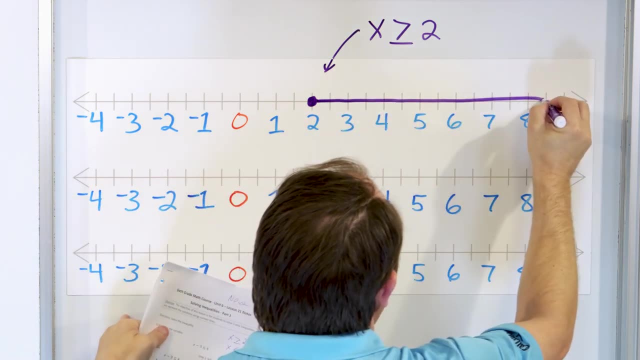 solid dot here to show that 2 is included in this, because it could be equal to 2.. But then what we do is we shade to the right, like this, And what you do is just kind of carry it on out as far as you want. You put a little arrow at the end. What this graph is really telling us is that if you're 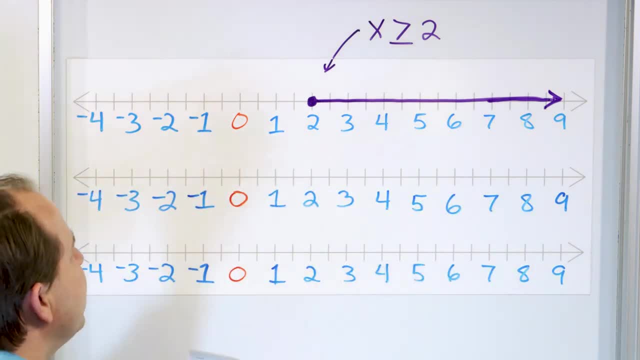 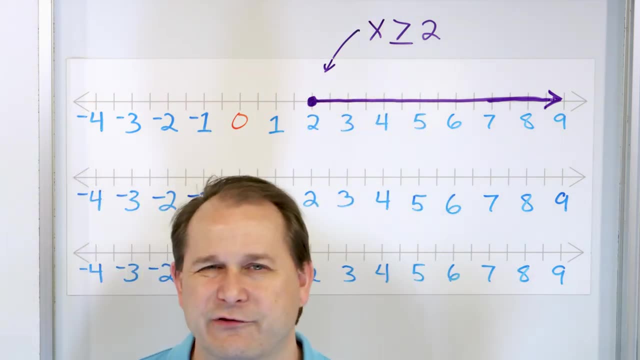 kind of came off the graph here a little bit. what this graph is telling you is: we're shading the number line. Anywhere in the shaded region on this number line is what this inequality represents essentially. So before, if I told you x is equal to 4, you just put a dot on the number. 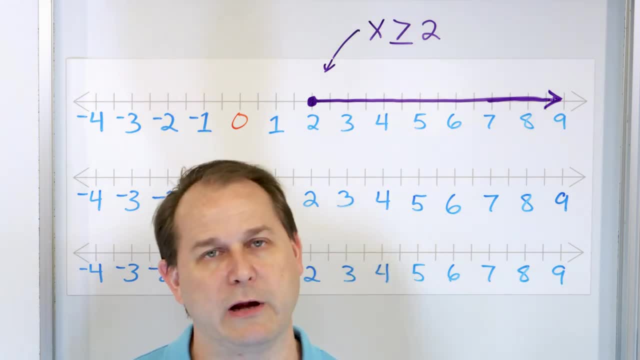 line. If I tell you x is equal to 3, you just put a dot on the number line. But if I tell you that x is greater than or equal to 2, then you have to put a dot on the number line at 2, because we have 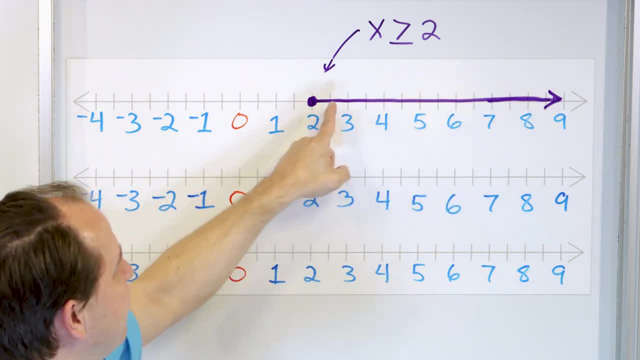 the equal sign here as well, But the shading tells you any number bigger than 2 as well is what x can be. And also I have the whole numbers here: 3,, 4,, 5,, 6, 7, but all of the numbers between: 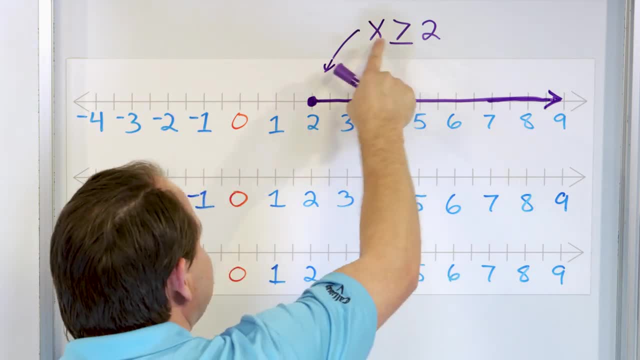 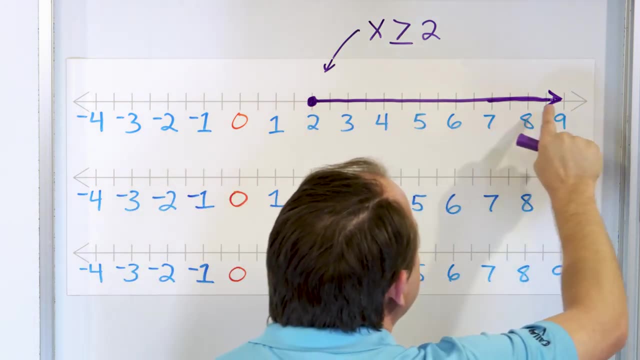 for instance, 3.5 is right here, x can be 3.5.. 4.67923 is a decimal somewhere around here. Any decimal that exists between these whole numbers, larger than 2 or equal to 2 is included in the. 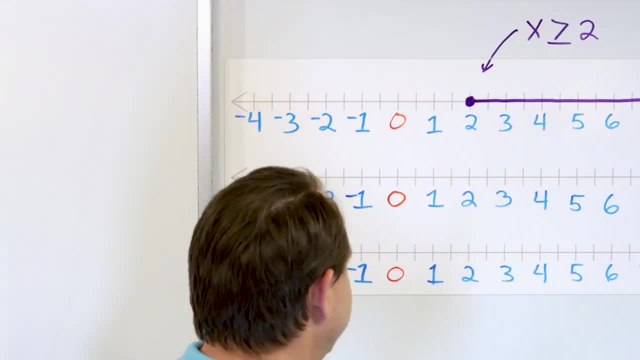 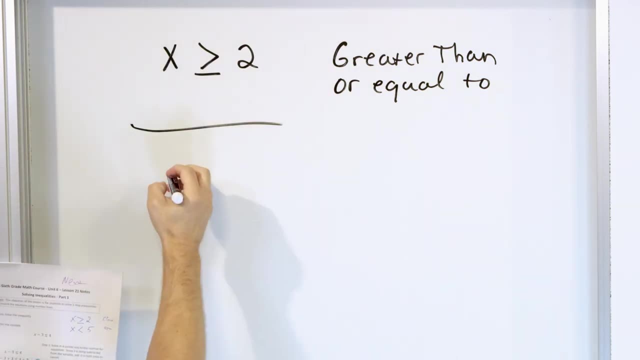 answer here, when we say inequality, x is greater than or equal to 2.. Let me show you one more, and then we'll actually solve our first inequality. What if we turn the arrow around? What if we say x is less than 5?? Now notice, here I don't have an 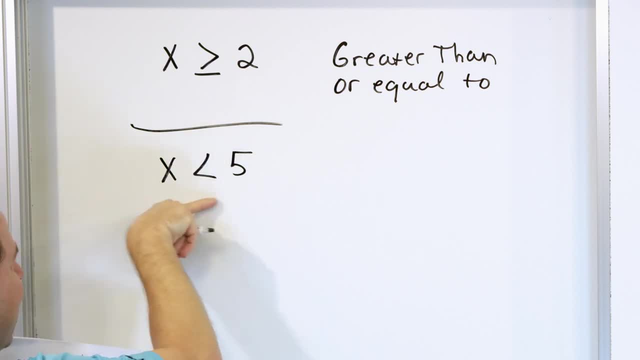 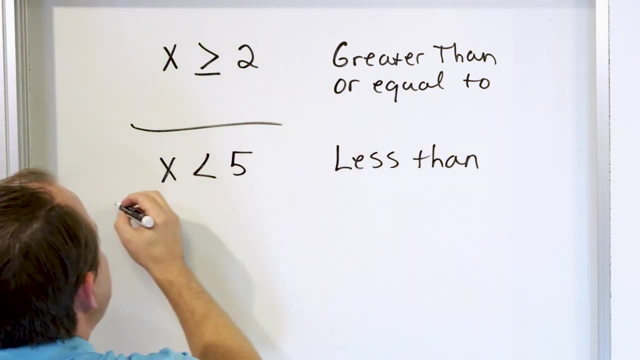 equal sign. here I just have a less than symbol. because we read left to right and we encounter the pointy end first, This is read as less than right. It's not equal to right because I don't have a little equal to bar underneath it. So what I'm saying here is: x can be any value less than. 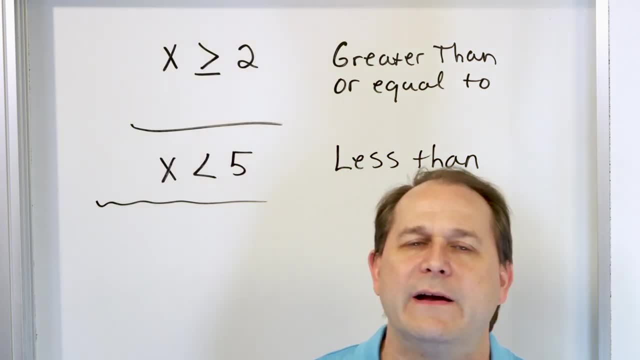 5,, but not equal to 5.. Less than 5,, but not equal to 5.. In other words, 4 is included but not in the possible values, because it's less than 5, right 0 is less than 5.. Even 4.999 is. 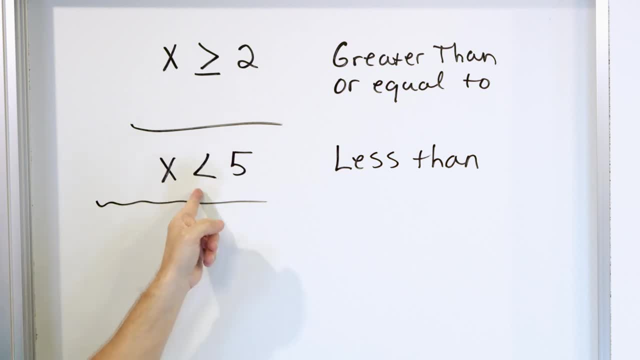 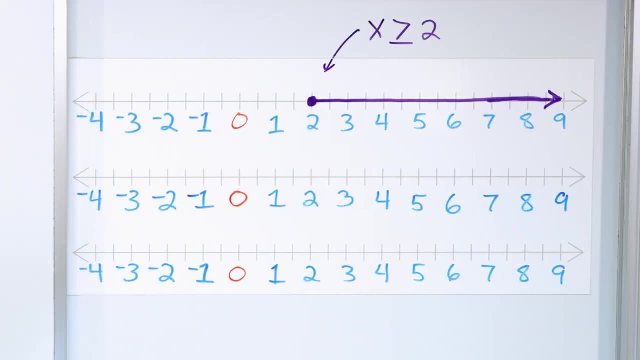 less than 5.. So it works and it satisfies this, and it's part of the numbers, but 5 itself is not part of the solution here. So what we can do is we can graph that as well. right, We can go over. 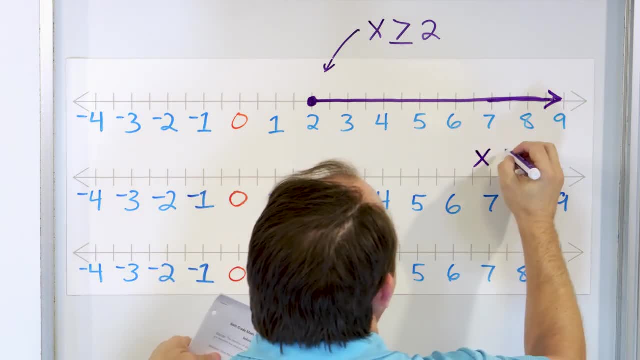 here. I'm just going to write this right here: x is less than 5.. This kind of line goes with this right here. But notice that there's no equal sign here: x is less than 5.. x is less than 5.. x is less. 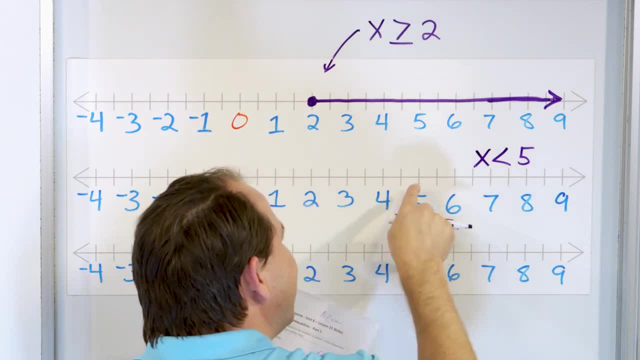 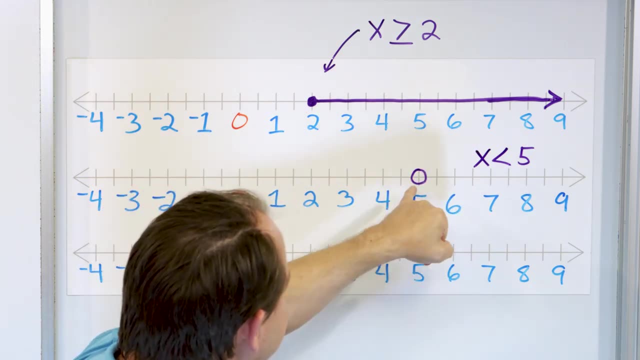 than 5.. So we don't want to put a solid dot here, because 5 is not really included. What we do is we put an open circle here on the number 5.. The open circle tells you that it's centered on 5,. 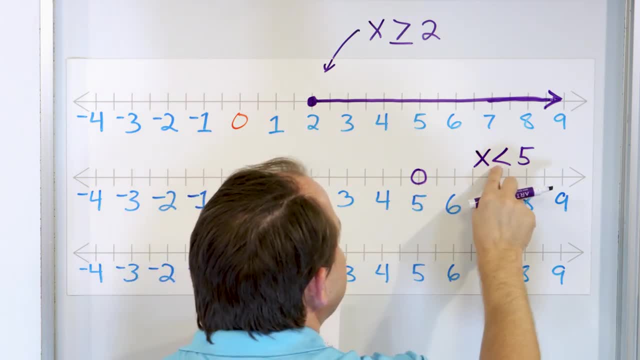 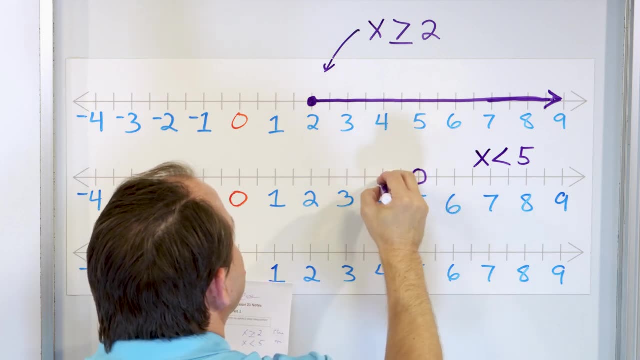 but 5 itself is not included here. But we still shade all of the numbers. But notice how the numbers are going the other way, because it's numbers less than 5. So it's all of the smaller numbers. So you kind of get over here and just do your best to do some shading. You can carry it as 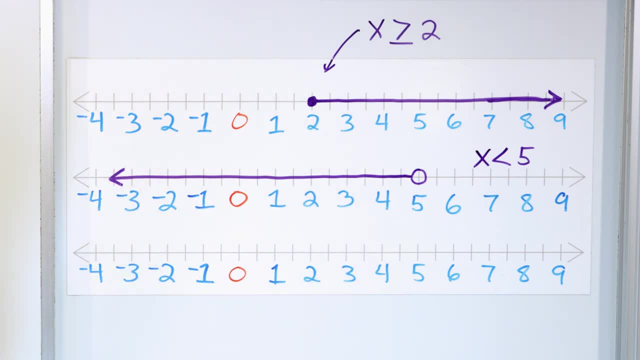 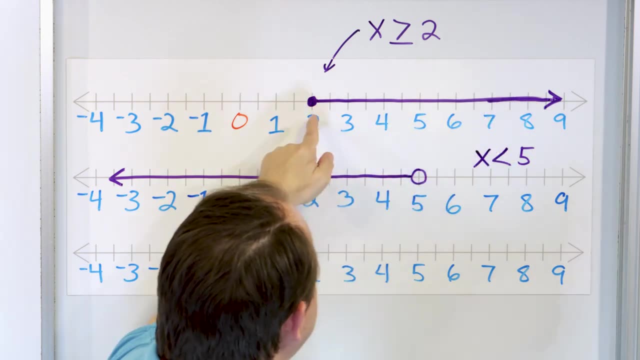 far as you want, put a little arrow and call it a day. So a couple things I need to make sure you understand. When the arrow points to the right, when x is greater than something, then the shaded region goes to the right past the number. When the arrow points to the left, it's just all values. 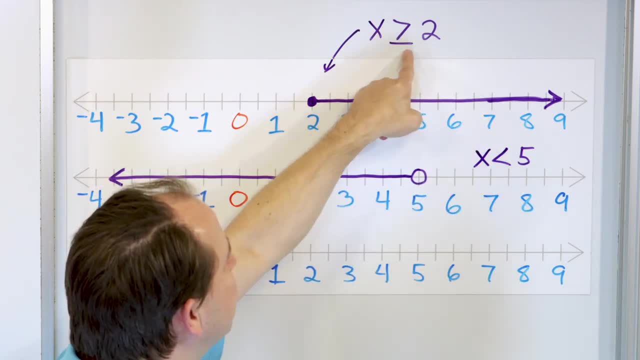 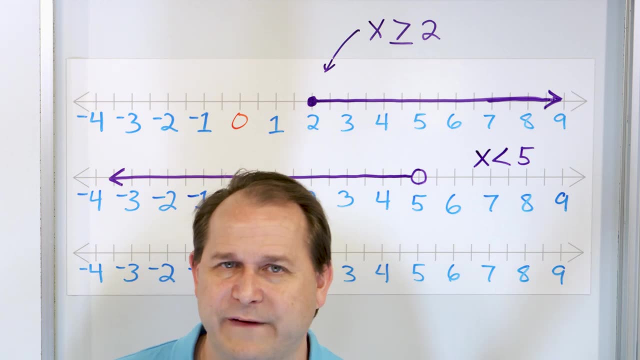 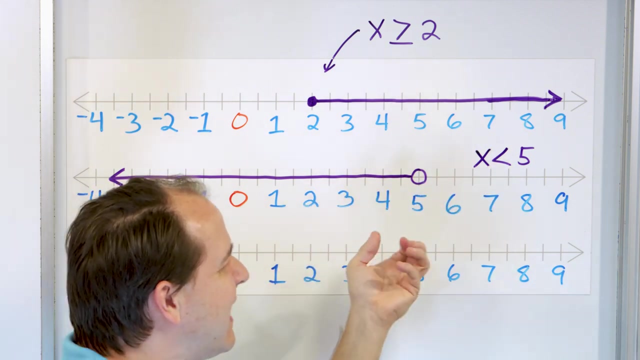 less than the number. And then if you have an underline underneath as well, you have to make the dot solid, because that number also is included in the possible values of x. That's what it means: greater than or equal to 2.. But when there is no line underneath here, then of course it's not. 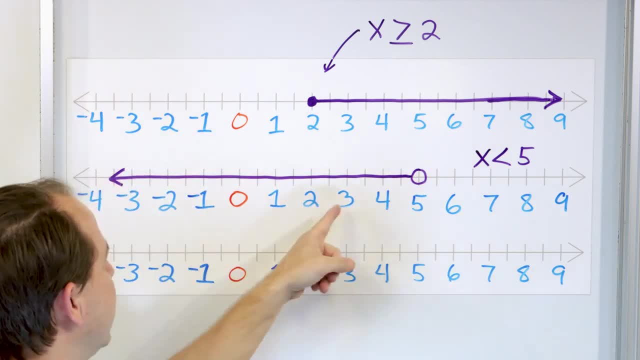 equal to 5.. It's just x less than 5.. So 4 is less than 5.. So x is greater than or equal to 2.. So 4,, 3,, 2, 1, even 4.5,, 4.7, those are all okay, Just 5 itself. the exact number 5 is not. 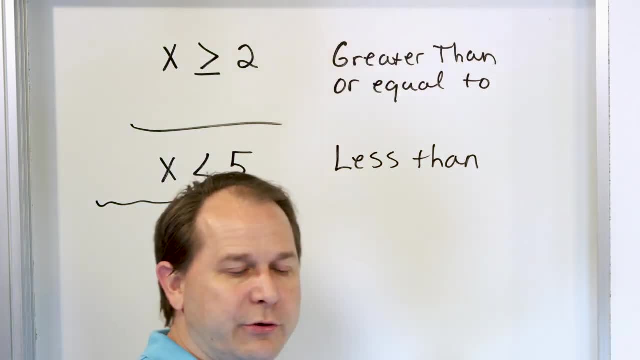 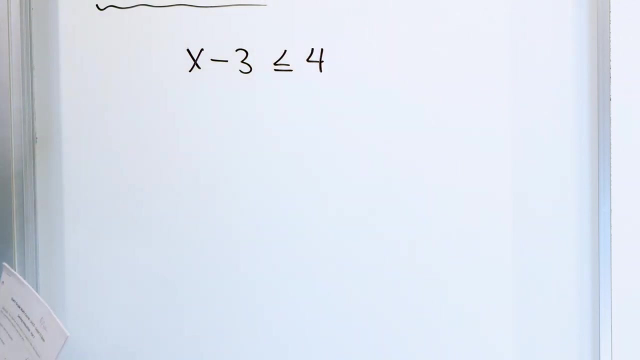 included. So what I need to do now is show you our first inequality that we're going to solve. So here we're just kind of graphing them and trying to understand it. Let's take a look at our first actual problem. x minus 3 is less than or equal to 4.. All right, So notice that this. 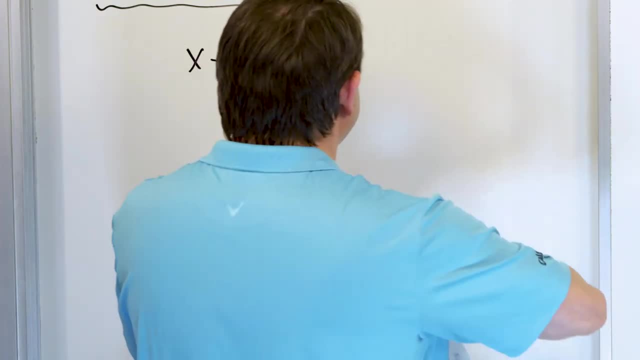 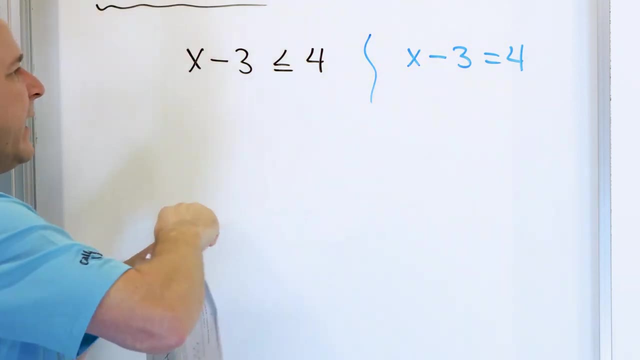 looks very similar to an equation. The equation version of this, if it was an equation, would be: x minus 3 equals 4.. Now you already know how to solve this right, Because this is an equal sign and we know that we can do whatever we want. So we would add 3 to this side and we would add 3 to 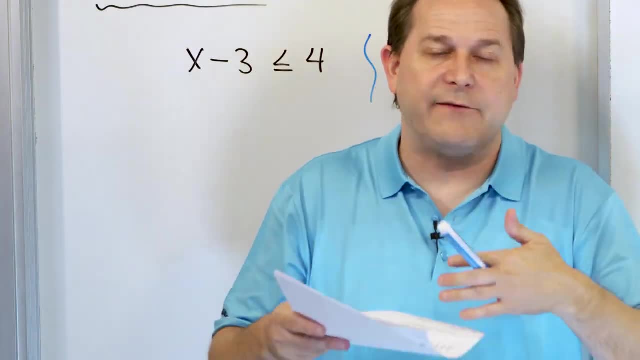 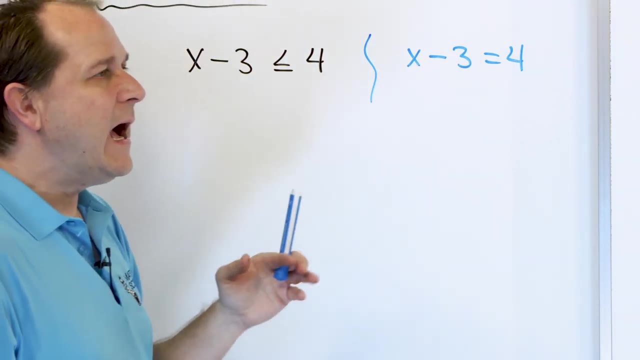 this side And as long as we do it to both sides, we keep it balanced and everything's fine and we get a value for x. So what we're going to do for the inequalities is: I want you to just pretend it's an equal sign. I know it's not an equal sign, but ultimately it's an equal sign. So I'm going to. 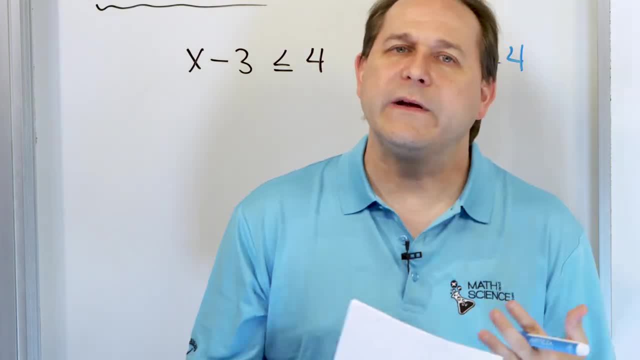 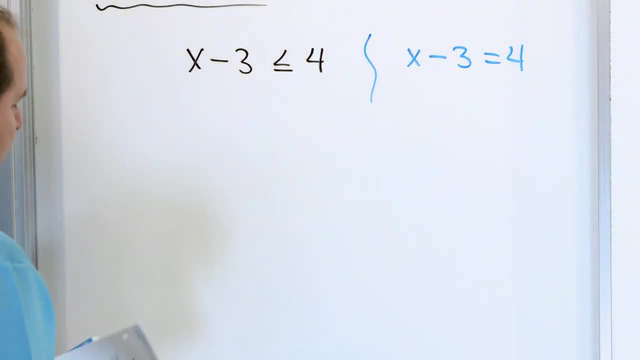 ignore it and just pretend it's an equal sign. We're going to solve the equation the exact same way that we always solve equations. We're going to apply that to this inequality because the rules are the same. I have one exception, I'll show you in a second, but the rules are basically the same. 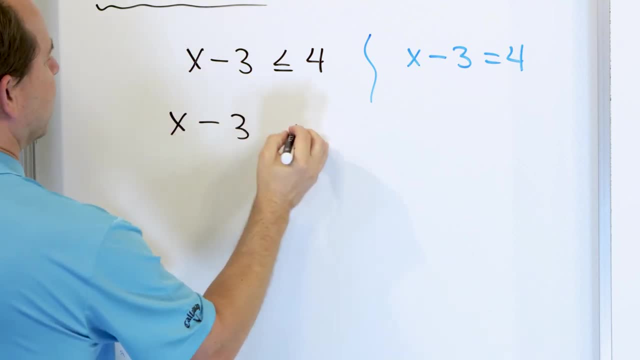 So let's go ahead and rewrite the problem, as we always do. All right, like this. Now what do we have going on on the left Again: pretend this is an equal sign. Pretend there's no arrow here. just an equal sign. 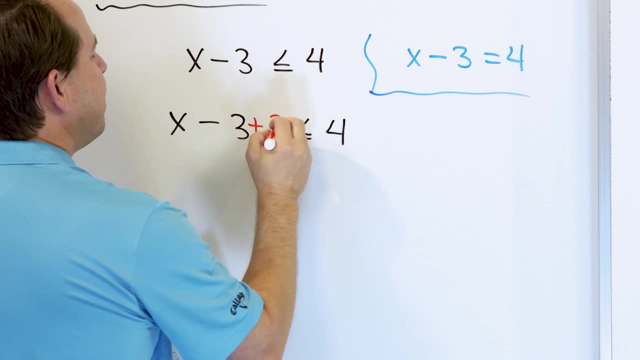 We have a minus 3.. So we want to do the opposite of that by adding 3 to the left, And to keep it balanced we have to add 3 to the right. You see, the rules are the same as for equations. 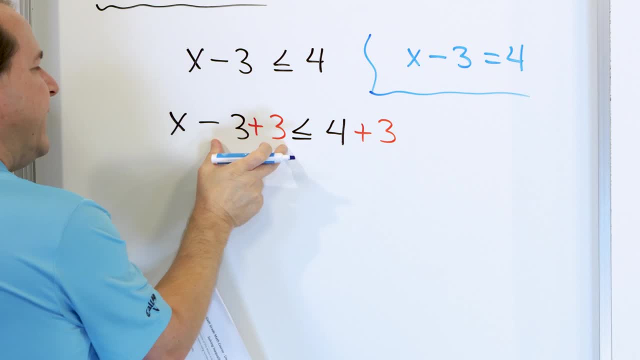 And then we have minus 3 plus 3 and they cancel out to give you 0. So all you have on the left hand side is x. This symbol stays the same. It's pointing the same direction. All of it is the same. 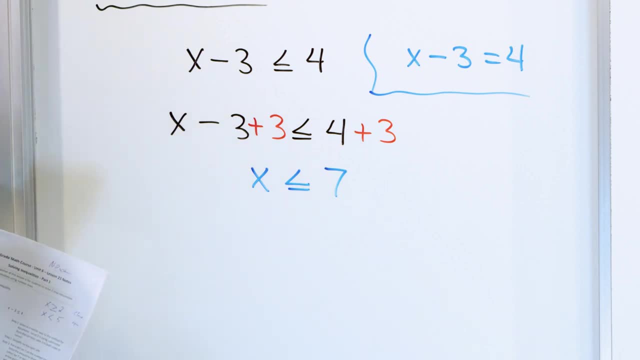 And then 4 plus 3 is 7.. So 4 plus 3 is 7.. So what we have figured out is that x has to be less than or equal to 7.. So we're going to explain a lot more about what this actually means, But first, before we do, 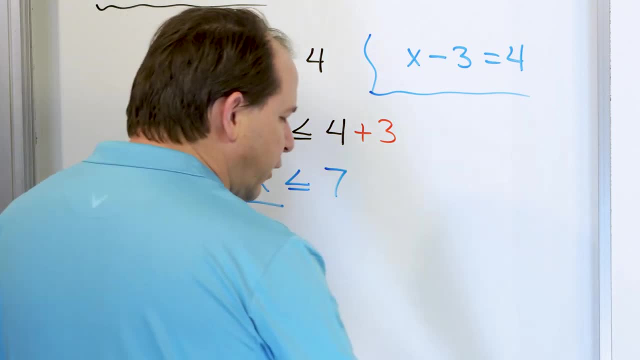 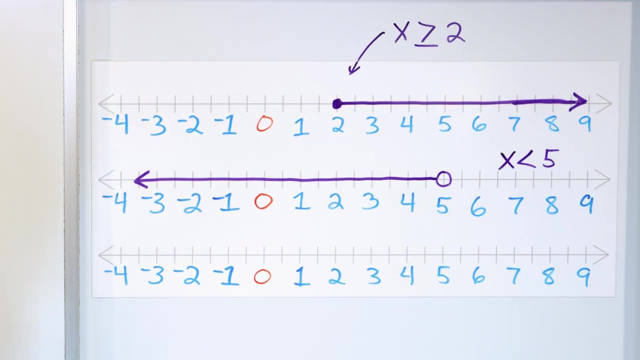 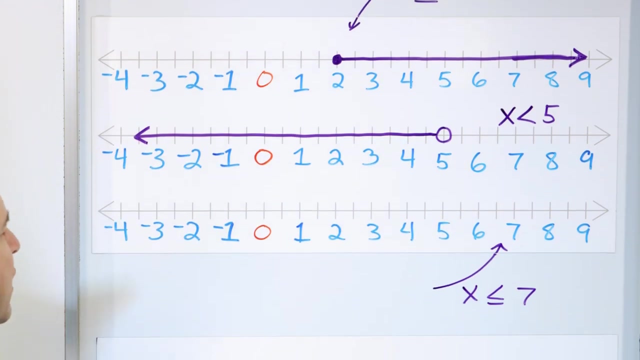 anything else. I want to graph the answer to this thing. So let's go over and remember: the answer to this problem is x less than or equal to 7.. So I'll write it right here. It'll be kind of right here: x less than or equal to 7.. That's the answer, right? So notice that there is an equal. 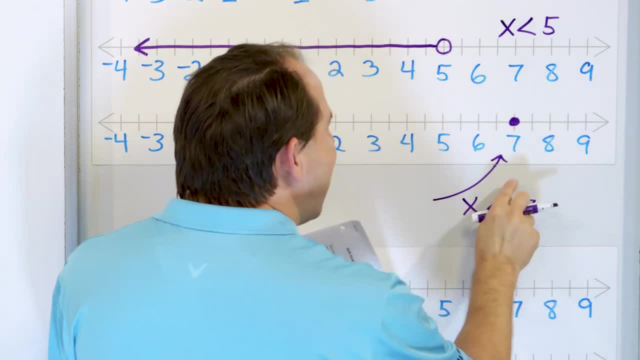 sign here. So we go to the number 7 and we put a solid dot here And we have a less than or equal to, which means we shade to the left All numbers less than 7.. So we go to the number 7 and we put a. 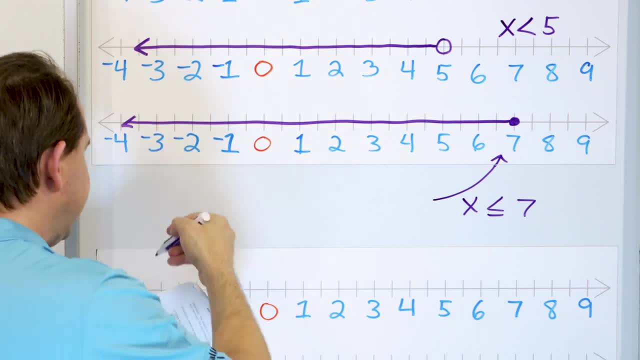 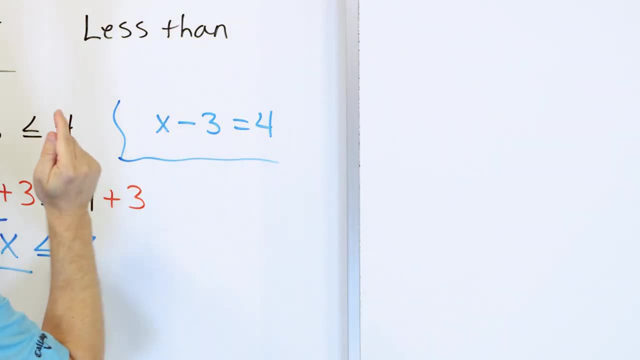 less than or equal to 7.. So what this means is, when you have an equation like the way I wrote it down in the first part right here, when you have an equation, there's only one value that's going to work in this equation And the number that's going to work is going to be 7.. Because if you 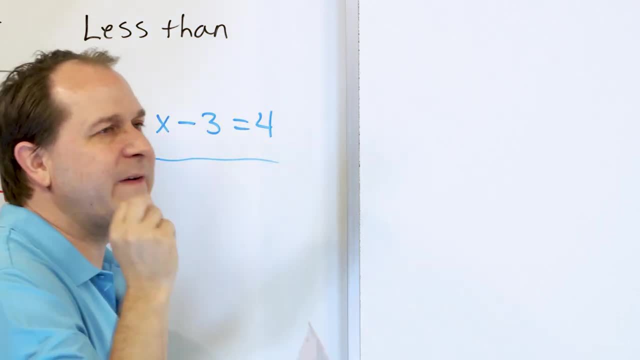 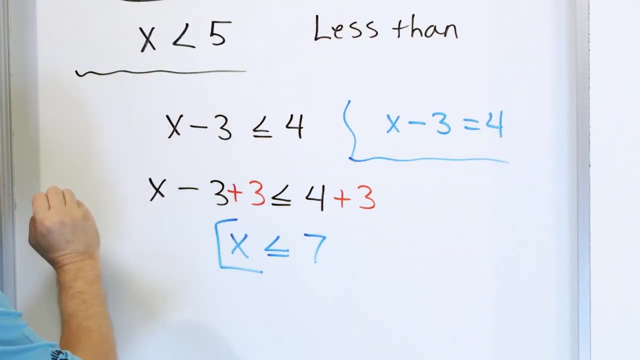 put 7 in here: 7 minus 3 is 4.. There is only one value for these equations that work, that make the answer work right, But when you have an inequality, there's actually an infinite amount of answers that work here. What answers have we got? What answers have we got? What answers have? 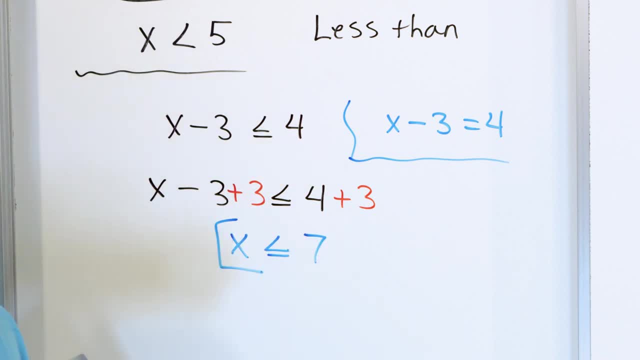 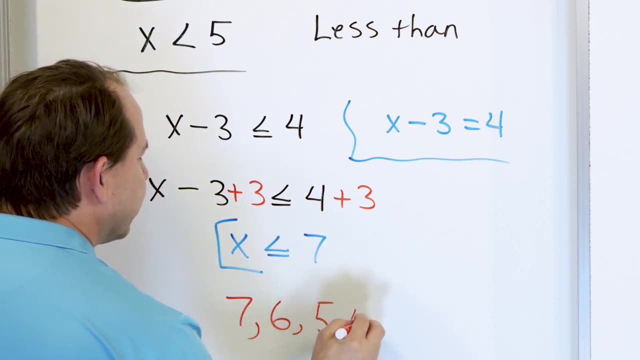 we decided on from this. Well, it has to be less than or equal to 7.. So that means that 7 works And anything less than 7, right, 6 works, 5 works, 4 works, 3, 2,, 1, 0. And then you go to the. 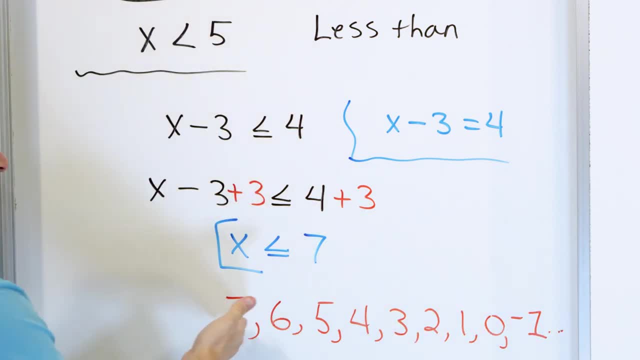 negative numbers, They also work too. Dot dot, dot, right. So there's literally an infinite amount of numbers that work in this original inequality. The solution is telling me: anything less than 7, but equal. So let's pick a value. Let's say 5.. Let's put 5 in here. 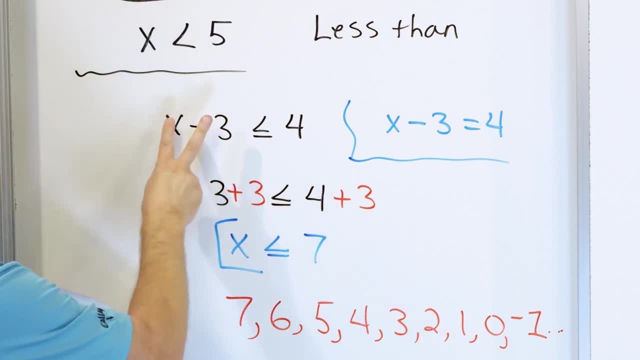 If you put 5 in for the answer, 5 minus 3 is what? 2. And 2 is less than or equal to 4.. So it works. What about the number 3?? Let's put 3 in here, 3.. 3 minus 3 is 0.. 0 is less than or equal. 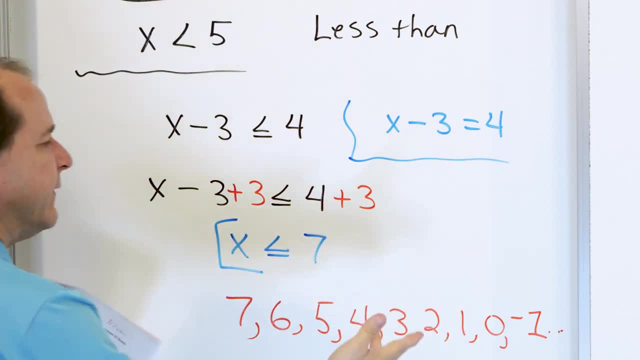 to 4.. And we haven't really gotten to subtracting negative numbers yet. But when you put numbers down here you'll get a negative number which is also less than or equal to 4.. What if you put the number 7 in? 7 minus 3 is 4.. So 4, is it less than? 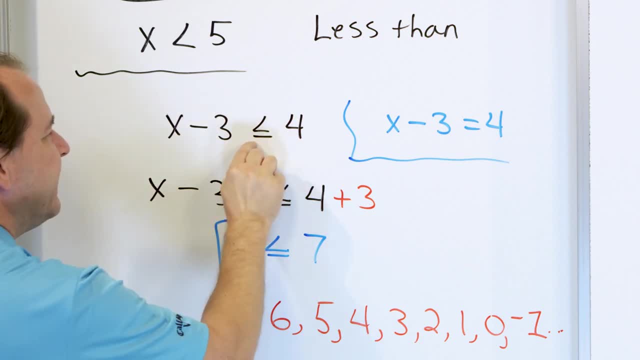 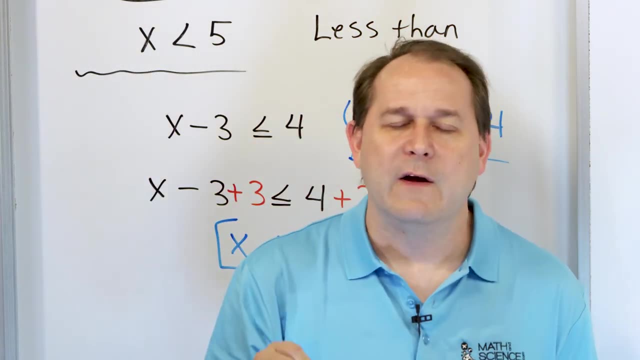 Or equal to 4?? Yes, because 4 is equal to 4.. And notice that this is an equal symbol as well. So what an inequality is is just replacing the equal sign with an inequality symbol. You completely ignore the symbol and use all the regular rules of solving equations. 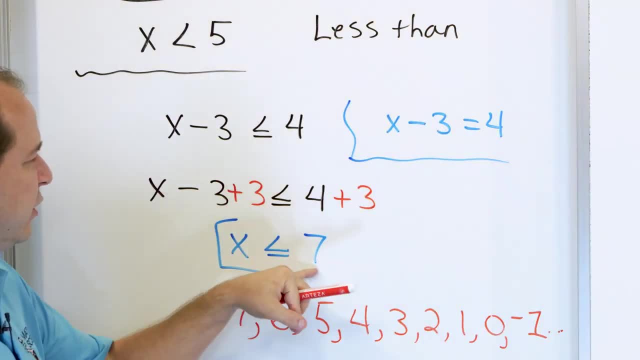 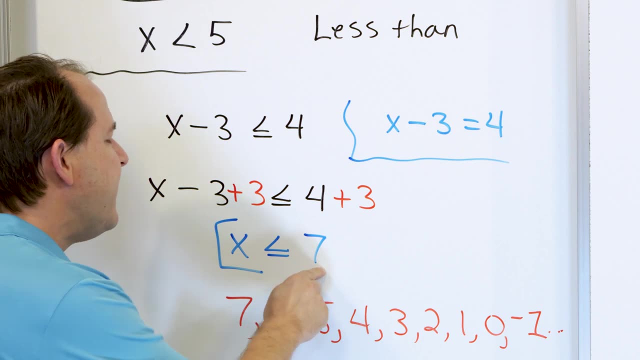 doing everything to both sides until you finally get it into what it looks like to solve an equation. But instead of an equal sign, you have this symbol here that you read as x is less than or equal to 7,, which means there's an infinite number of numbers that we can put into the 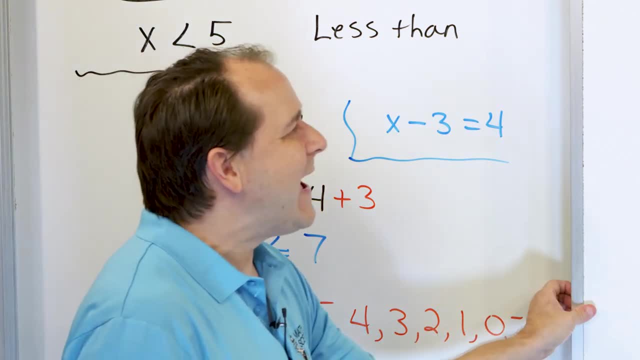 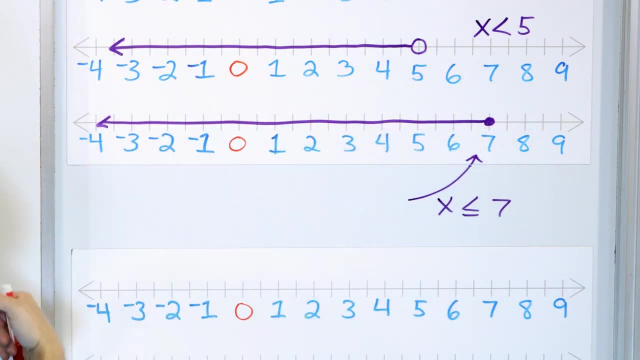 equation and still satisfy the inequality. And when we graph it visually, what it's basically telling us is the number 7, plus all of these numbers to the left off, to negative infinity. they all work when I put them in there. So we're graphing the solutions, Because you can just look. 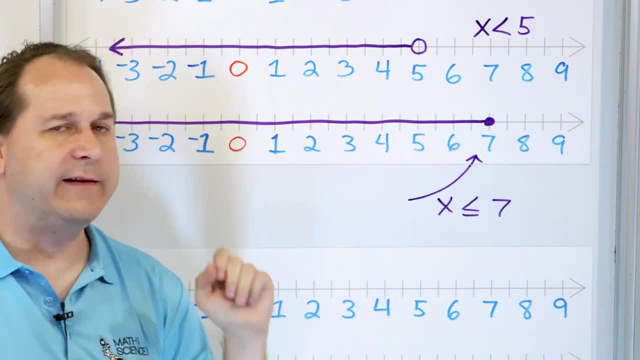 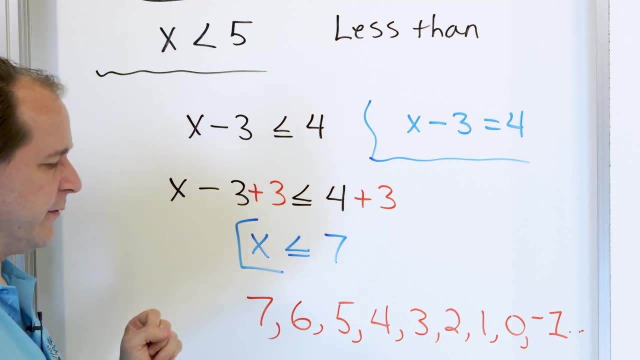 at the graph and anywhere you see a shaded thing here, and if there's a dot, that number works as well- counts as a solution. All right. Now there is one gotcha I want to talk about before we finish solving all the problems, And that is: I told you that we used the same rules of the world. 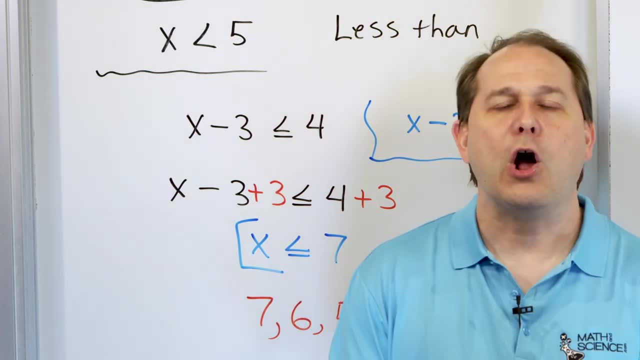 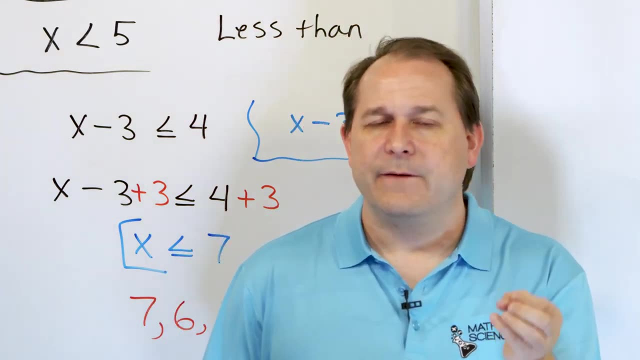 Same rules of solving equations for inequalities. That is true, All of these are going to involve adding and subtracting, So it's going to be quite easy once we get the hang of it. But if, when you're solving inequality later on down the road, we're going to cover this a little more later, When. 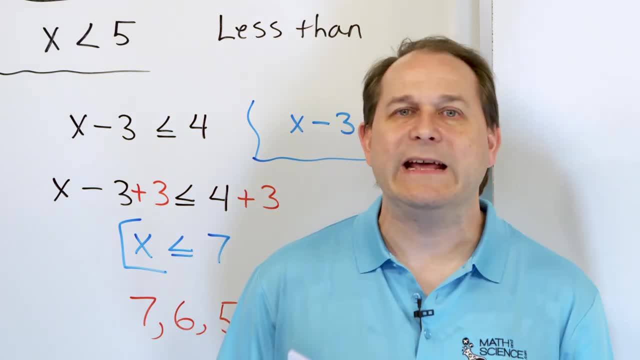 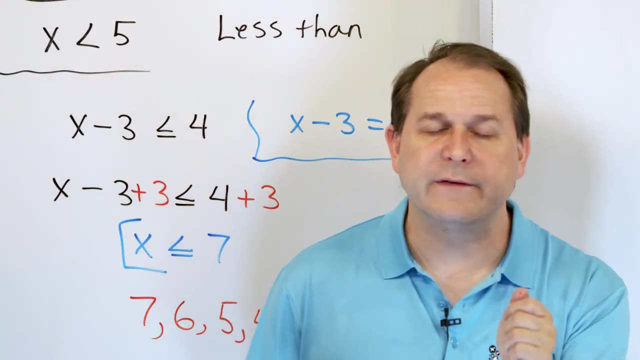 you're solving an inequality if you have multiplying and dividing going on. if you multiply or divide both sides of this inequality by a negative number. if you multiply or divide the inequality on both sides because you can do what you want, right. If you multiply. 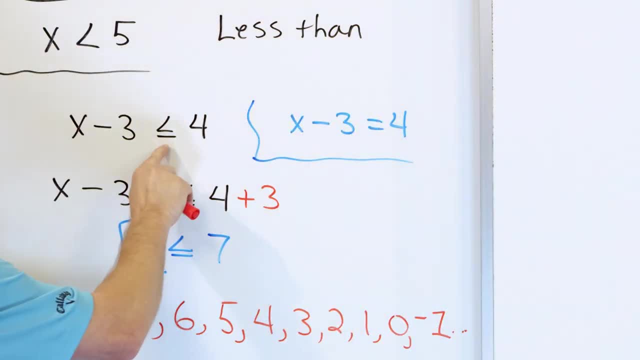 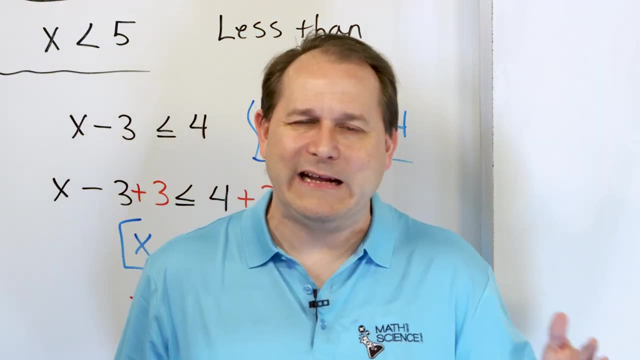 or divide by a negative number, then the symbol must flip the other way. The arrow points the other direction And I know that you might see that the first time, like why does that happen? I don't want to get into why it happens because it's not the focus of this lesson We're going. 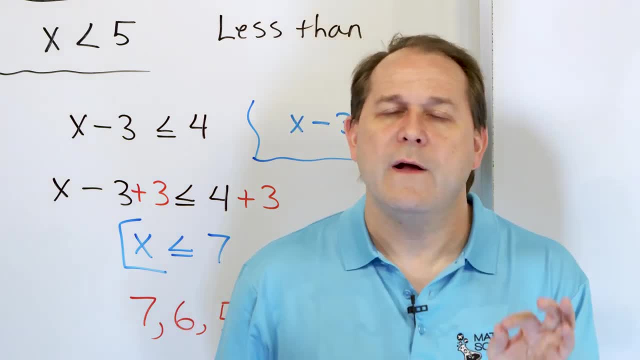 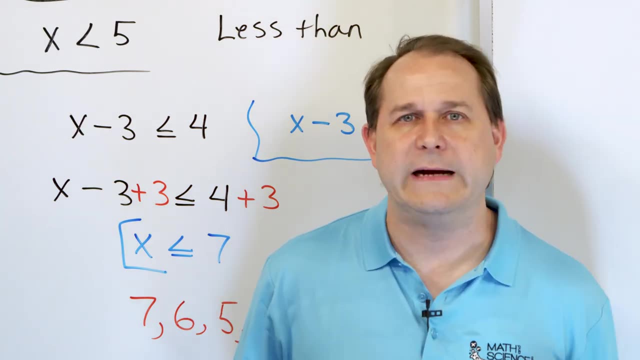 to get to it later and I'll explain it in great detail later, But I just want you to know that the rules of solving inequalities are exactly the same as solving equations. The only difference is, if you ever multiply or divide an inequality on both sides by a negative number, then the symbol 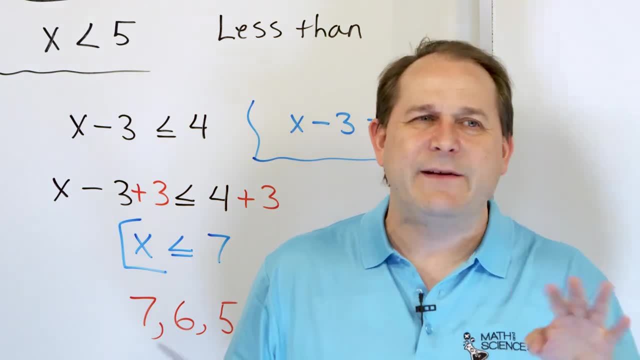 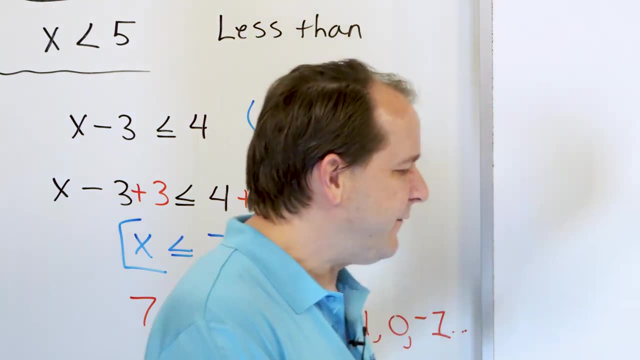 has to flip directions And that's because when you multiply by a negative it kind of changes the meaning of what the sign is. I'll get into it later, but that's why. But for this lesson we're not going to actually have any of those problems, so I don't want to focus on it too much. 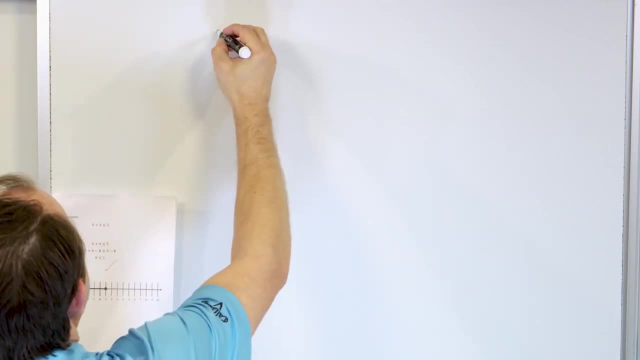 So now what I'd like to do is crank through and solve more problems. Let's say we have: h plus 4 is less than or equal to 5. So what we do is we completely ignore and pretend this is an equal sign. So we just rewrite it: h plus 4.. Give ourselves some space, We're 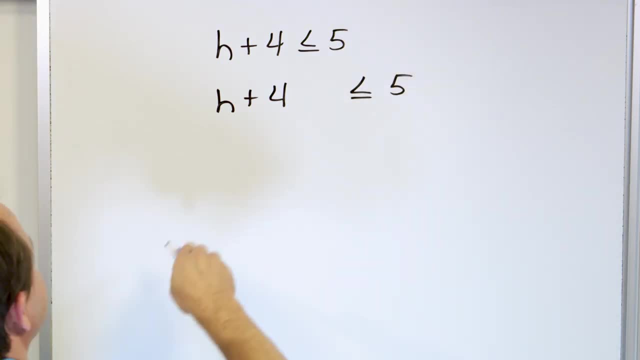 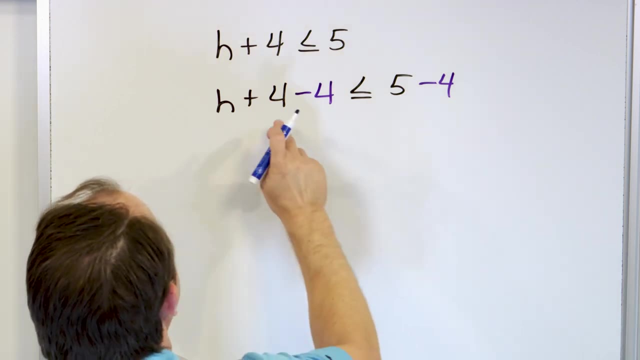 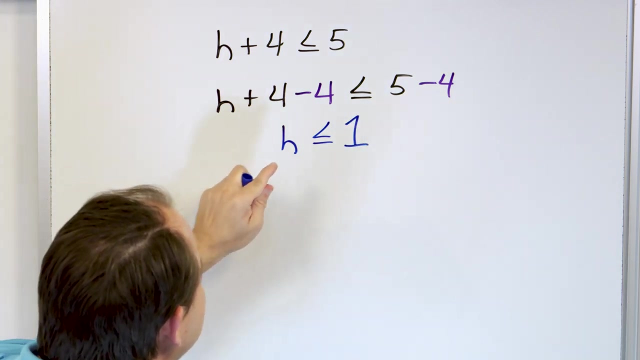 going to get rid of the 4.. We'll subtract on both sides. The only thing that will be left on the left-hand side- because this is 0, is h. The inequality symbol comes down, and 5 minus 4 is 1.. So what we are saying here is that this value of this variable can 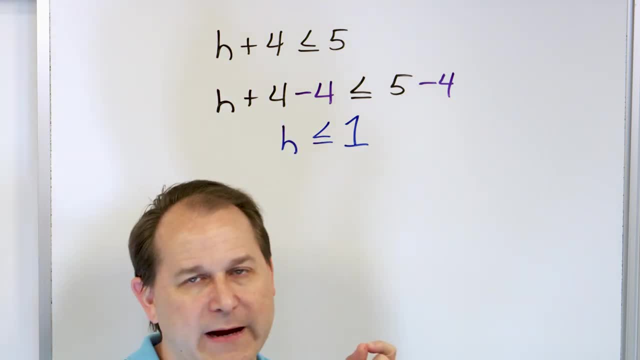 be anything less than 1, but it also can be equal to 1, right? So let's pick something less than 1.. Let's go with 0, because that is less than 1, right, Put 0 in here, 0 plus.